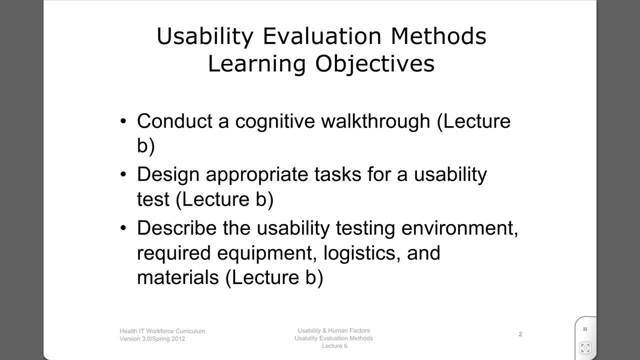 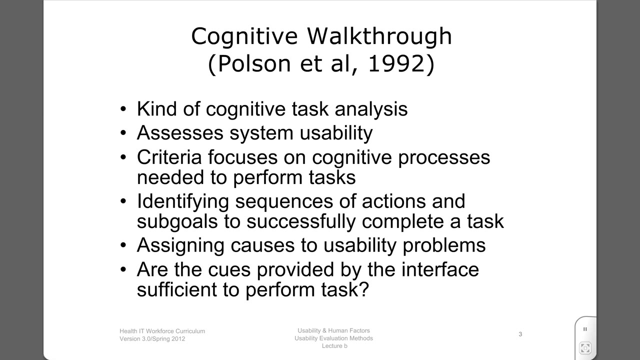 One of the objectives is to understand how to develop a protocol for usability testing and undertake various kinds of analysis. In addition, one should be able to describe the usability testing environment, including the required equipment, logistics and materials. The Cognitive Walkthrough- CW- is an alternative usability inspection method. 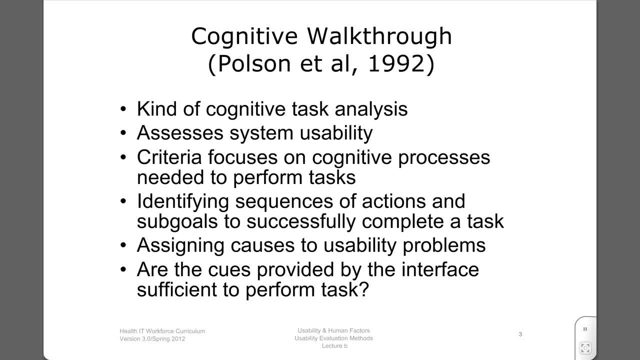 It is richly steeped in cognitive theory, most notably Don Norman's Theory of Action. The analysis takes the form of a Cognitive Task Analysis CT and a CT-A. In a minute or so we will go through the procedure, and then I'm going to illustrate this method with a couple of examples. 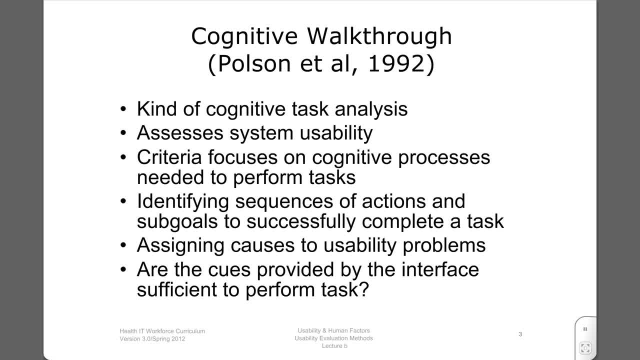 Criteria of the analysis focuses on cognitive processes needed to perform tasks. It involves identifying sequences of actions and sub-goals to successfully complete a task and assigning causes to potential usability problems. The key question is whether the cues provided by the interface are sufficient to perform the task. 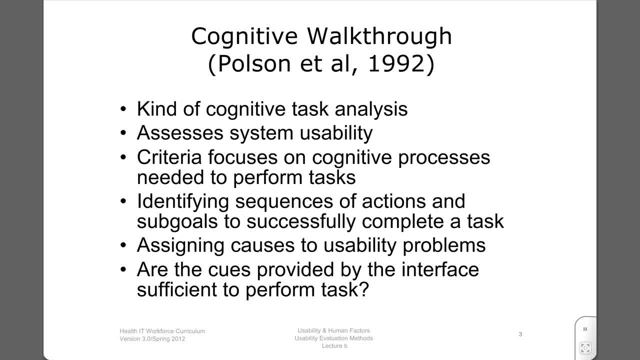 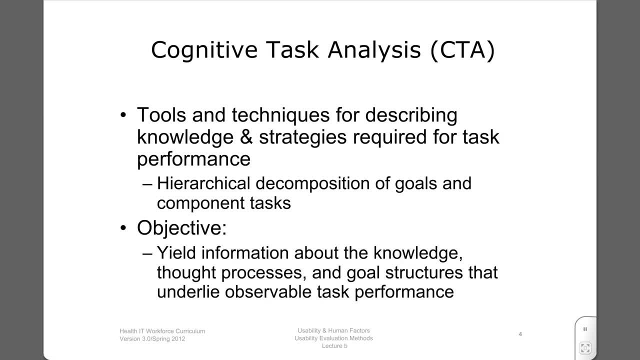 The alternative is that the user will have to wander through a more complex space, expending greater time, effort and cognitive resources. The CTA is a family of methods for describing the knowledge and strategies required for task performance. It involves a hierarchical decomposition of goals and component tasks. 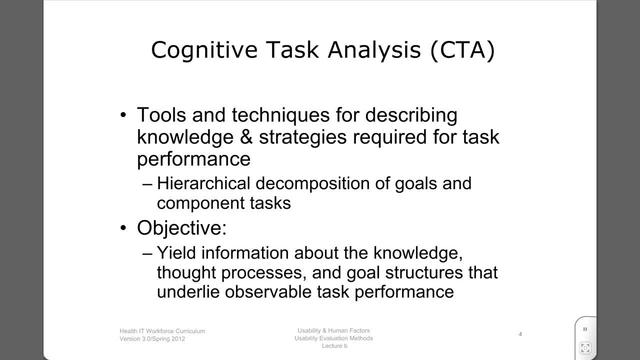 For example, performing a Google search can involve the following two components at minimum: 1. Selecting key terms and 2. Evaluating the results of the search. Each of these components has distinct goal-action structures. This should become much clearer in a couple of moments. 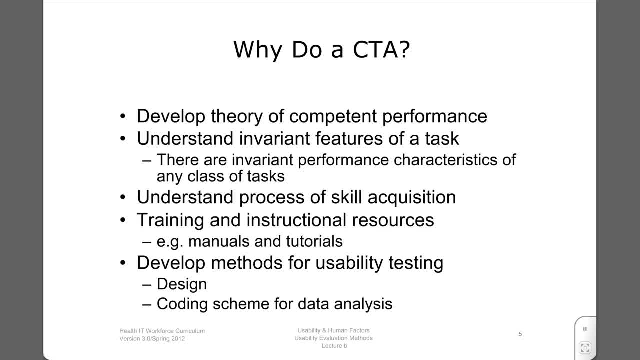 There are a wide range of reasons for undertaking such an analysis. For example, you can develop a theory or model of competent performance for a task or classes of tasks Using the above example. there are a set of skills and knowledge needed to do a good job. 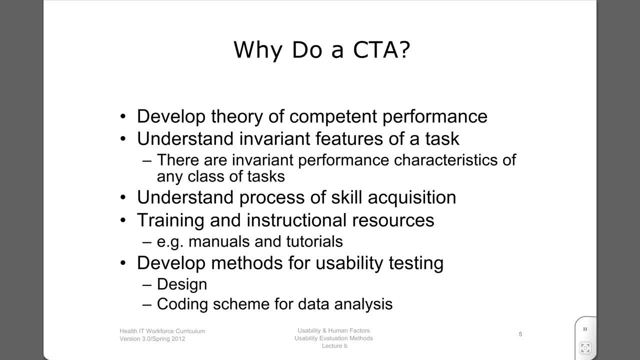 The CTA can help us to arrive a model of how to do that competently. The CTA can also be used as a means to develop training materials. Although usability inspection methods are stand-alone methods, they can be used in concert with usability testing. 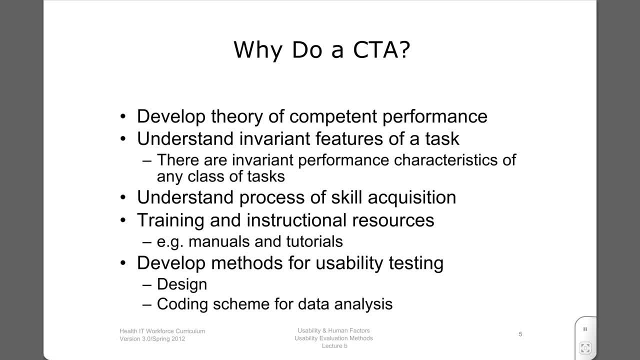 The CW is a very good precursor to usability testing. You can use the analysis to develop a set of tasks to give to users. One can also differentiate between complex and less complex tasks. One common and relatively simple measure of complexity is the number of steps or actions needed to complete a task. 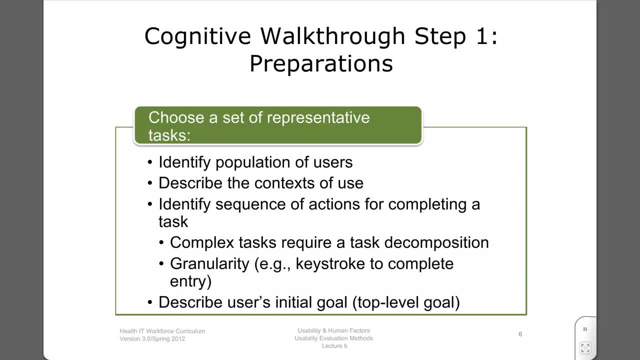 There are three essential steps to perform a CW. There are a number of decisions to be made prior to undertaking the analysis. This begins by identifying the inputs to the CW, beginning with a selection. The CW is a relatively time-consuming process and it is important to judiciously select representative tasks of interest. 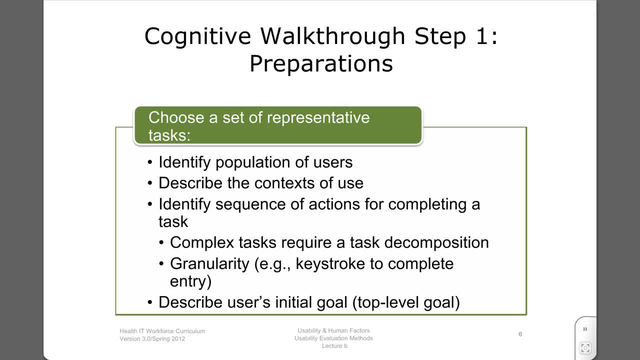 For example, an electronic health records system may support hundreds of different tasks, But these tasks can be grouped into a relatively small, finite set of tasks, including data retrieval, data entry and ordering of tests. One may select two or three tasks. It is important to keep a target population in mind. 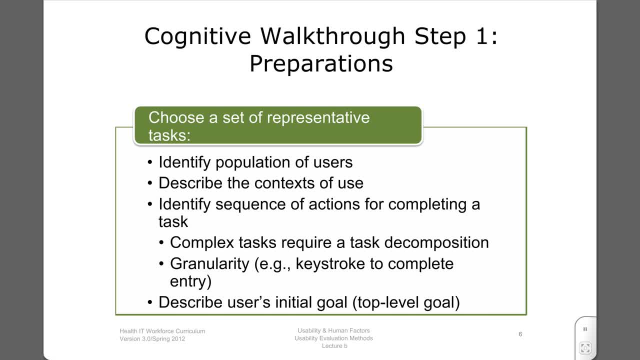 Will the target population be relatively sophisticated computer users, or will they include some novices? Will older adults also be expected to use the system? Granularity of analysis is an important issue to address. One may choose to do a very fine-grained analysis where the focus is on the keystroke level, for example. 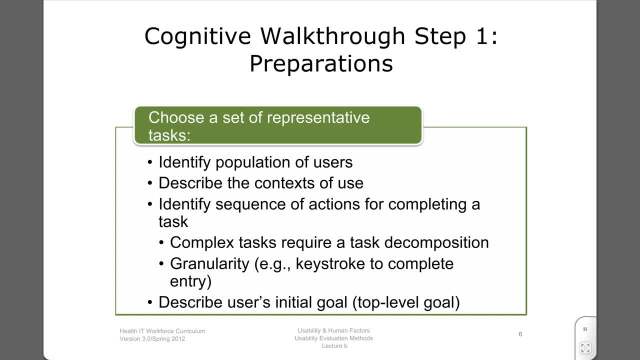 Alternatively, one may choose to conduct a higher-level analysis and focus on the types of errors and data entry. The less granular analysis may prove to be more useful in most practical contexts. It requires less time and expertise to analyze goals and actions and a higher level of abstraction. 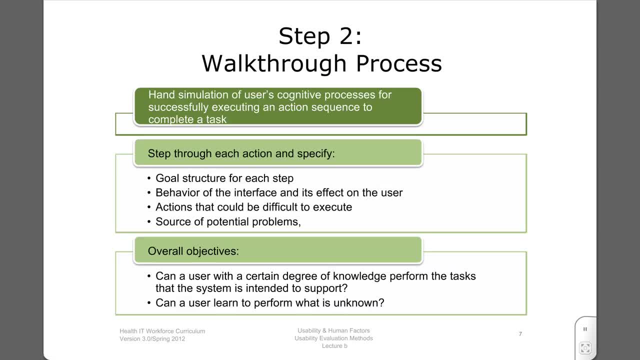 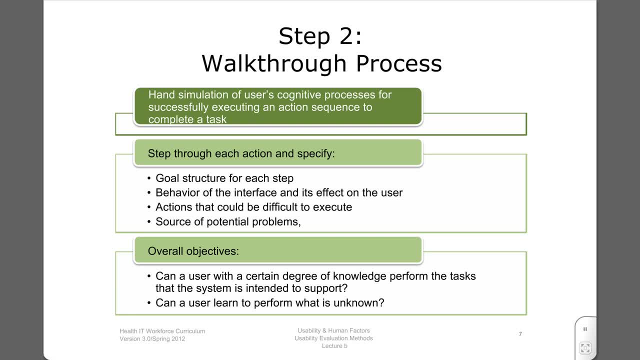 The analyst steps through each action and specifies: 1. Goal structure for each step, 2. Behavior of the interface and its effect on the user. 3. Actions that could be difficult to execute. 4. Source of potential problems. As mentioned previously, The overall objectives are to determine whether a user with a certain degree of knowledge 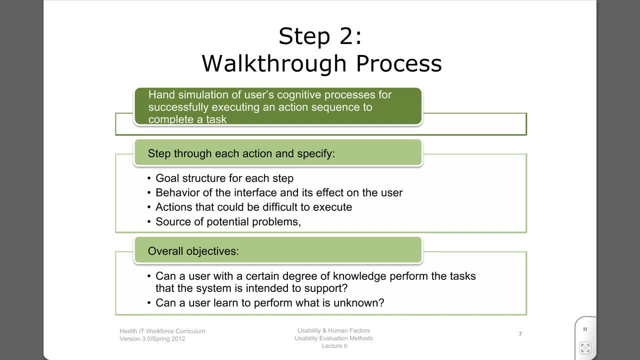 can perform the tasks that the system is intended to support. If not, can they readily learn to use the system? Learnability is an important issue when dealing with systems such as EHRs. Such systems necessitate a certain learning curve, and some are much easier to learn than other ones. 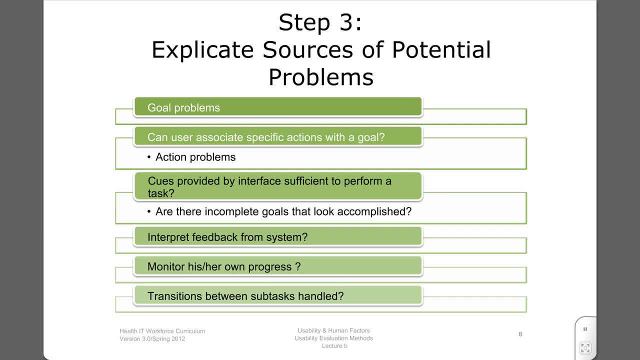 The third phase is to explain the sources of potential problems. For example, does the system provide sufficient feedback after every action or are there potential sources of confusion? Are the transitions between subtasks abrupt and confusing, or are they handled gracefully, keeping the user informed? 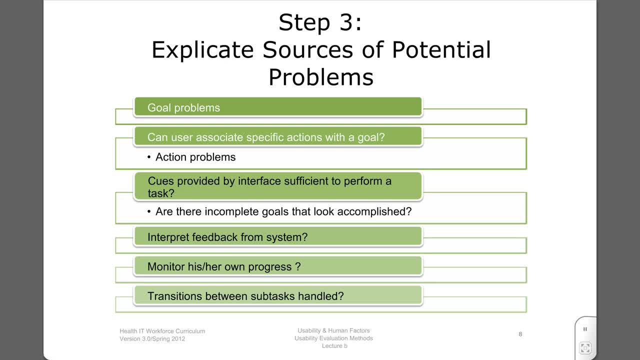 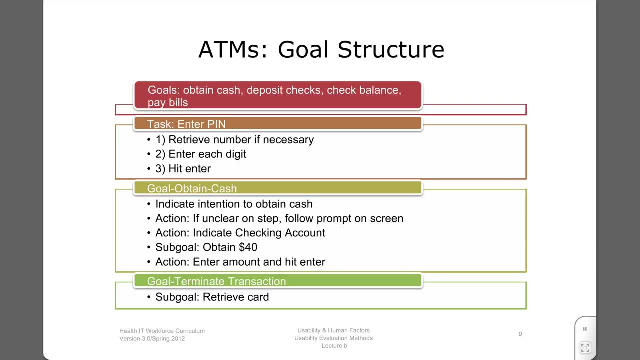 It is also helpful to draw Nielsen's principles to organize one's findings of potential problems. Our first example is using an ATM or automated teller machine. This slide provides the input to the cognitive walkthrough. ATMs support a handful of tasks such as obtaining cash, depositing checks and paying bills. 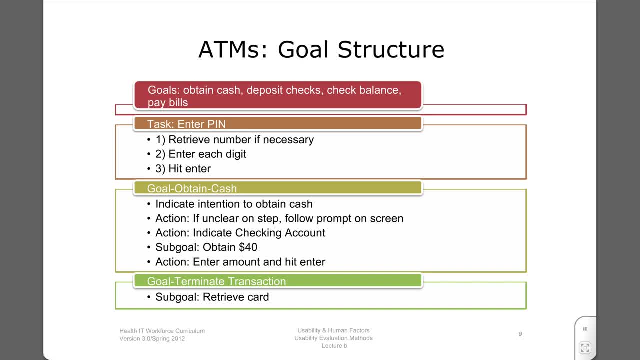 To execute one of these tasks, you need to carry out a set of steps. ATMs are walk-and-use technologies. No training is required. Almost everyone knows how to use one. at this point in time, This is a potential walkthrough of an ATM. 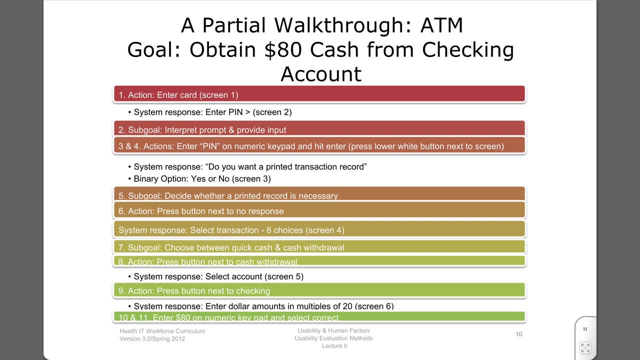 The task and the top-level goal is to obtain $80 in cash from your checking account. There are 11 actions displayed on this slide. The first action is to enter your card and the system's response is to prompt you to enter your personal identification number: PIN. 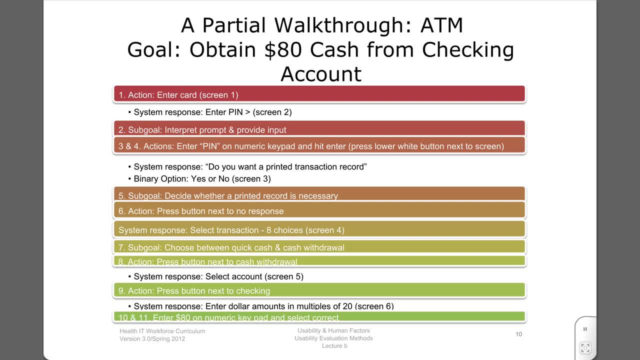 Subsequently, the interface presents you with a set of dialog screens in which you are expected to make certain choices. As you move through the actions in the walkthrough, you move closer to completing the top-level goal of obtaining $80 from your checking account. 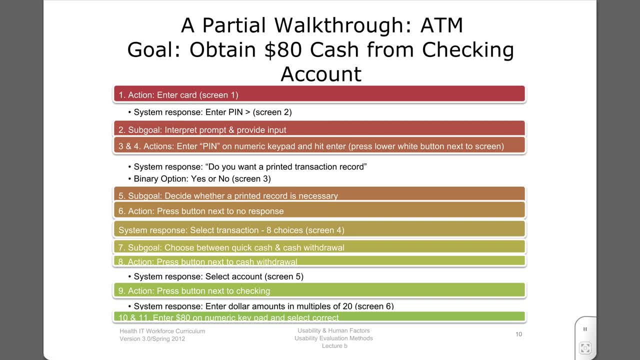 The interactions are rather straightforward. Each screen reflects a goal-action structure with particular sub-goals necessitating certain action sequences. In the walkthrough, you are expected to enter your personal identification number, PIN, and the sub-goal is to complete the task. 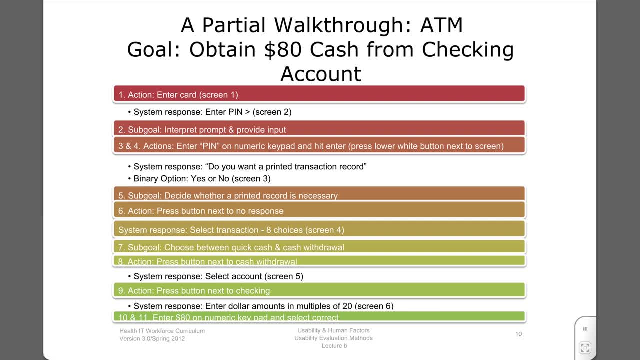 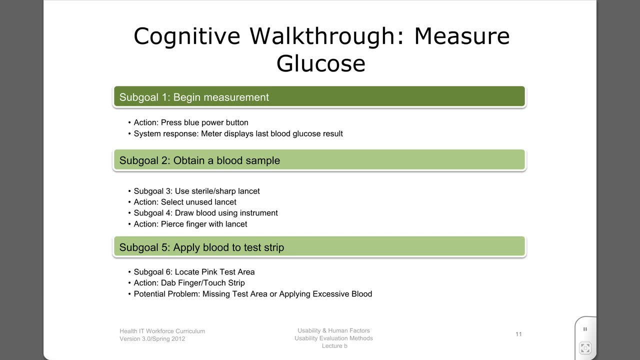 By the eleventh action the user should be entering $80 on the numeric keypad and selecting Correct from the offered options. We conducted a cognitive walkthrough of a commercial glucose meter. The CW can be used to evaluate any kind of device. A detailed but partial walkthrough. 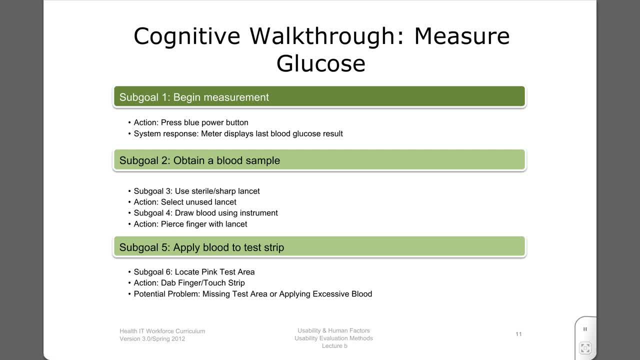 is illustrated over the course of the next three slides. The task was to measure glucose. This slide shows three sub-goals. Begin with a goal of beginning a measurement. Each top-level sub-goal, such as Begin Measurement, names a goal-action structure. 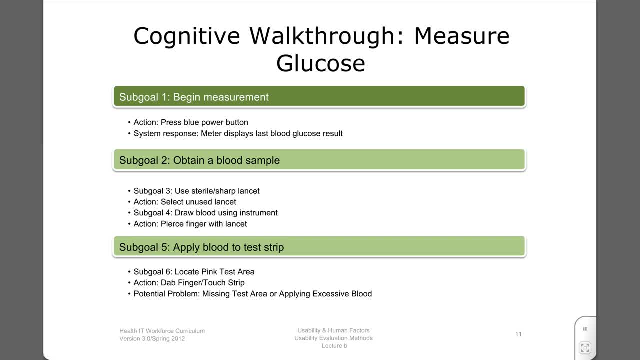 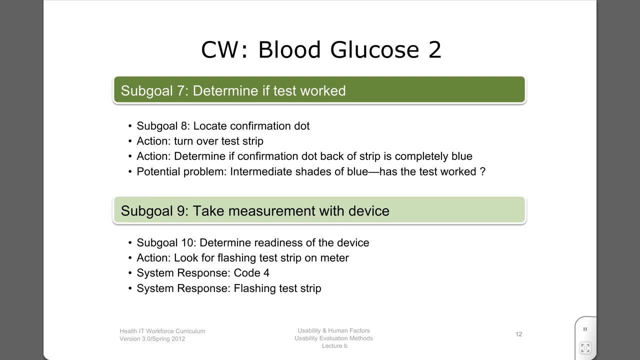 involving one or more actions followed by a system response. Although this is a very basic task, there are quite a few steps and the process is surprisingly complex. The sub-goals on this page continue to involve preparation to take the measurement, The system response of the flashing test strip. 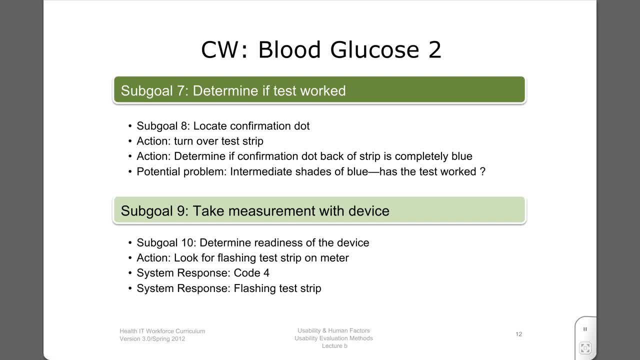 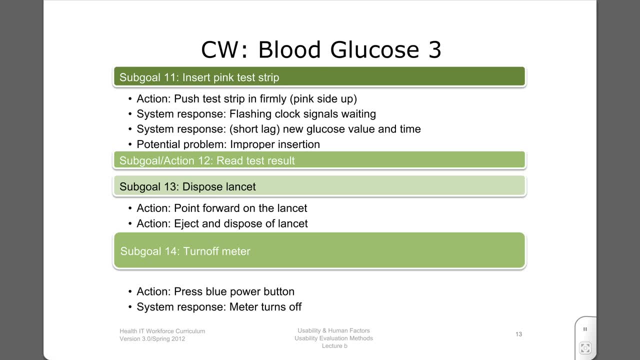 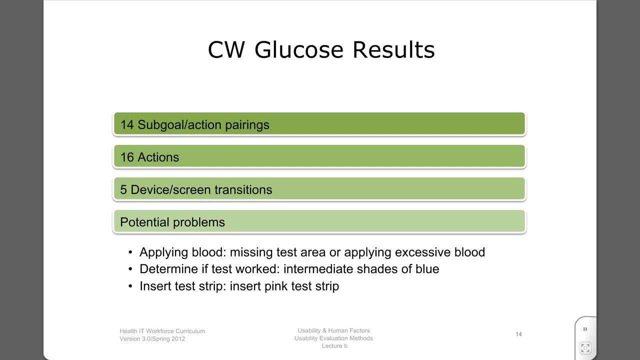 at sub-goal 9, signals that the device is ready to take the measurement. At sub-goal 12, the test result becomes available to the user. All together, this is the most basic of tasks. It necessitated 14 sub-goals. 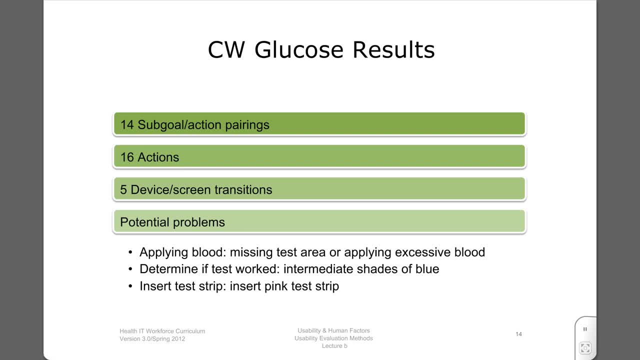 16 actions and 5 device-slash-screen transitions. We also identified a handful of problems that may make taking the test or interpreting the results difficult for some users. It should be noted that this is an older glucose meter and more modern ones may require fewer steps. 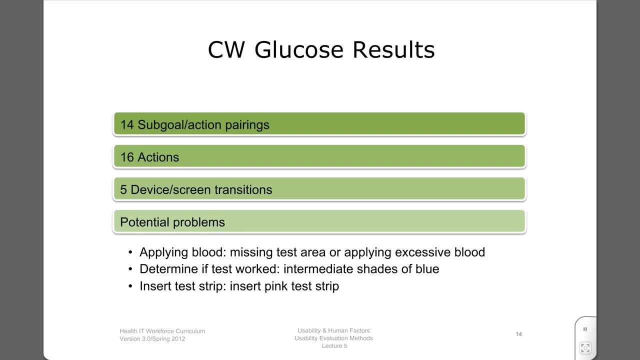 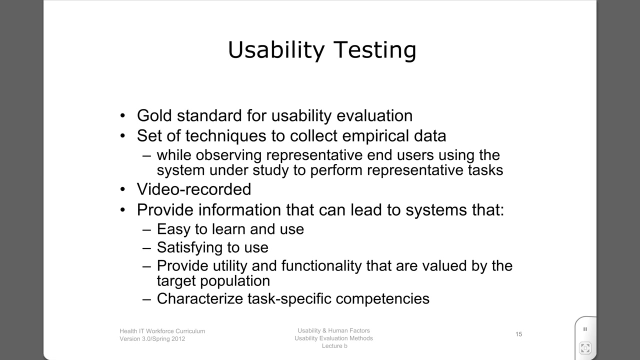 However, when you unpack a task into goals and actions, it becomes transparent that something that seems simple is actually more complex and may present challenges for some users. Our focus on this work was on lower literacy older adults. The final method to consider is usability testing. 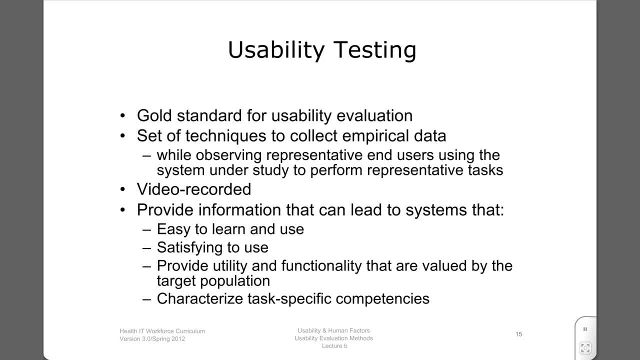 It is widely believed to be the gold standard for usability evaluation. The usability inspection methods involve the judgments and speculations of analysts. Interviews, focus groups and questionnaires are either subjective or involve self-reports. Usability testing provides hardcore evidence as to the nature of difficulties. 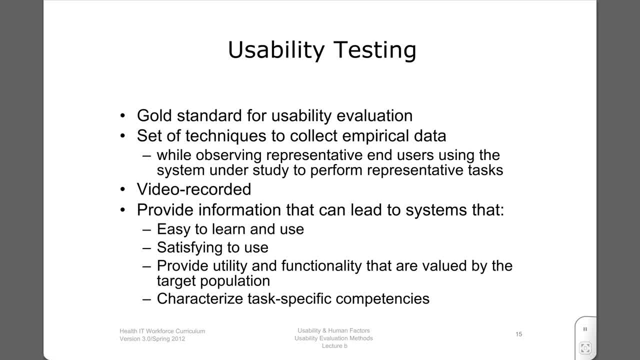 that users encounter when interacting with a system. We don't wish to disparage the other methods. All of the evaluation methods are useful. In addition, usability testing is the most time-consuming and costly of all the methods. Usability testing refers to a class of methods. 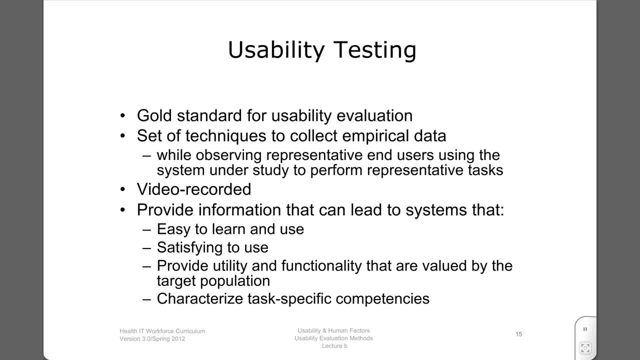 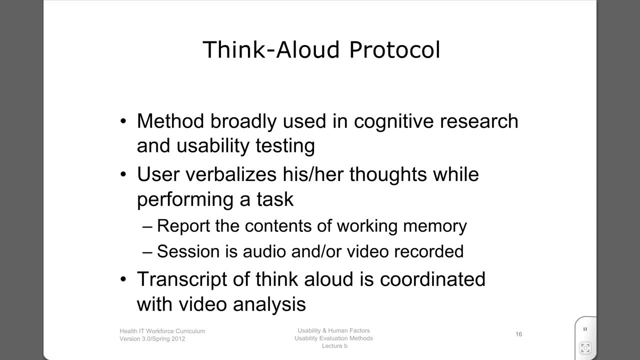 for collecting empirical data from representative users performing representative tasks. Some sort of video capture of users performing the tasks is typical. The think-allow protocol is a method broadly used in cognitive research as well as in usability testing. The user is asked to verbalize his or her thoughts. 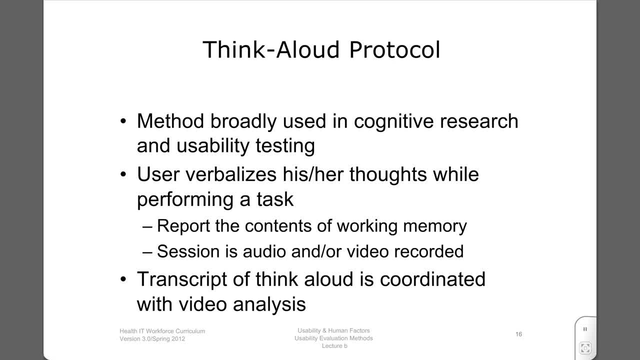 while performing a task, They are expected to report the contents of their working memory, basically whatever comes to mind as they perform the task. The user is discouraged from engaging in self-analysis, for example commenting on their strategies. The session is audio and or video recorded. 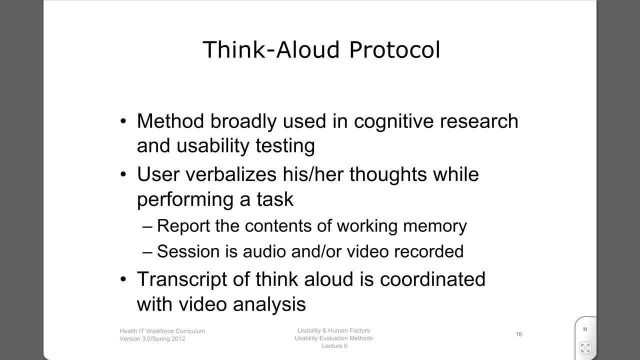 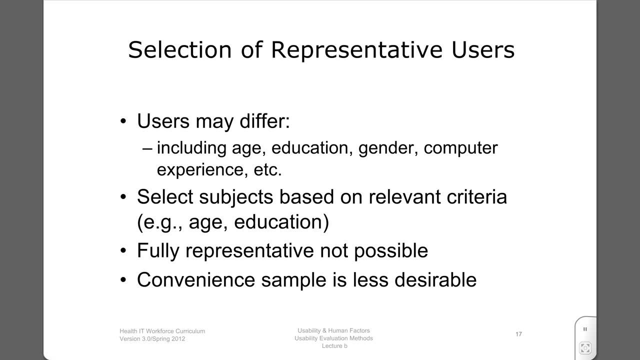 The transcript of the think-allow protocol is coordinated with video analysis and provides a rather complete picture characterizing the nature of the interaction. The selection of users for usability testing should mirror the overall population of users to the extent possible. For example, if you are testing 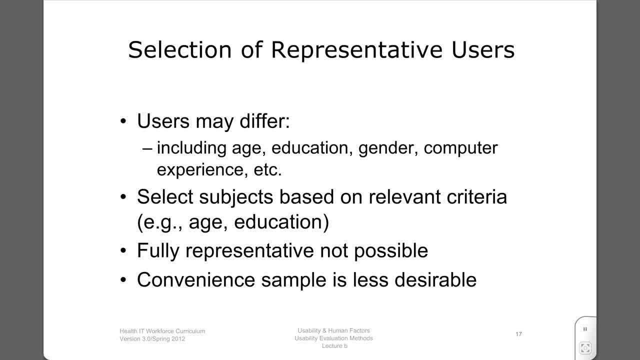 a glucose meter but don't include older adults in your sample, then you are discounting about 40% of the population who are likely to use the device. Usability testing involves in-depth testing with a small number of subjects: The heuristics. 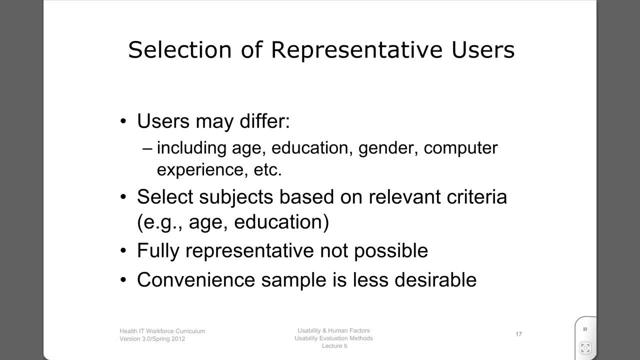 is that a test can be perfectly valid with as few as five or six subjects. In addition, five or six subjects may find upwards of 80% of the usability problems. A typical usability testing study will involve five to ten subjects. This small number- 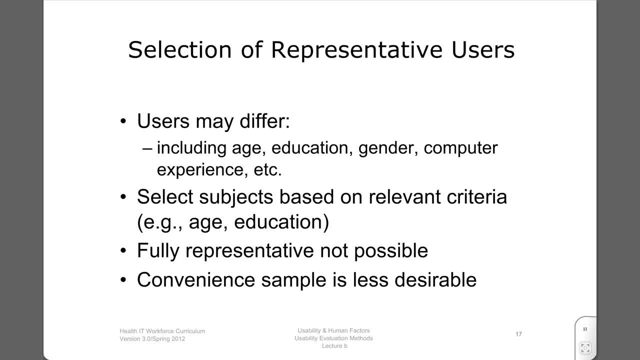 makes it difficult to get a fully representative sample. Convenience samples are very enticing. For example, they may include the more enthusiastic users. However, they are not likely to be representative of the overall population of users. This may lead to skewed results and lead to wrong conclusions. 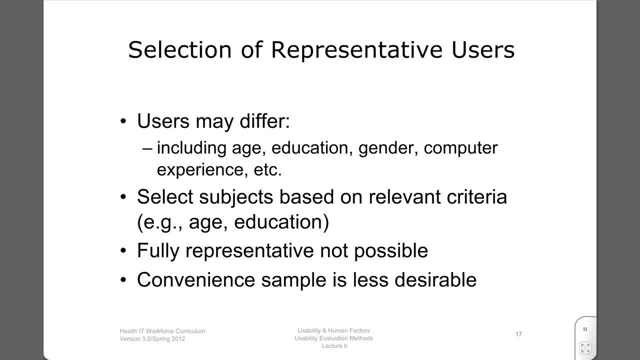 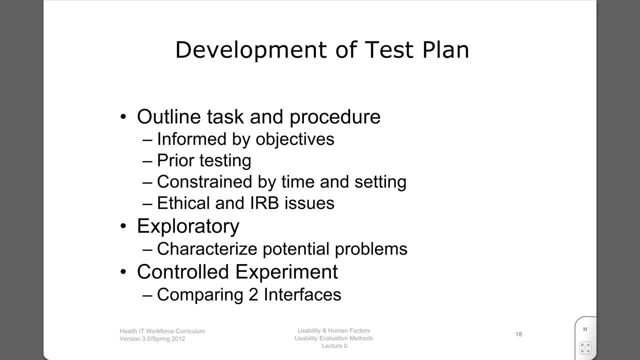 such as the system has relatively few usability problems. The test plan includes a crystallization of your objectives: What tasks are most important to test? It is advisable that a testing session not last longer than an hour as participants begin to get fatigued and frustrated. 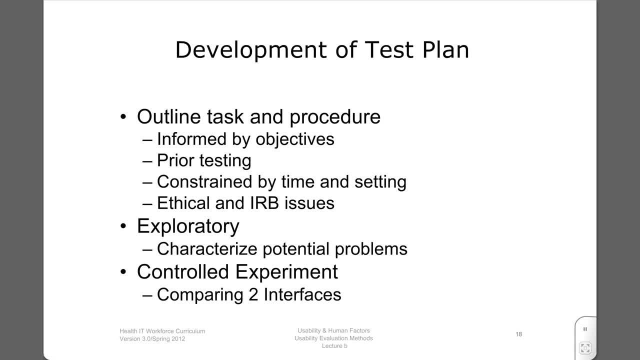 One also needs to select a sequence of tasks. Sometimes the order is unimportant. A general heuristic is to begin with the simpler tasks and progress to the more complex ones. If a subject is unable to complete an easier task, there is no reason to give him or her. 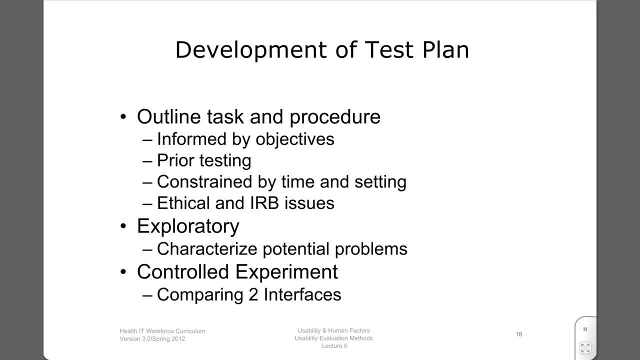 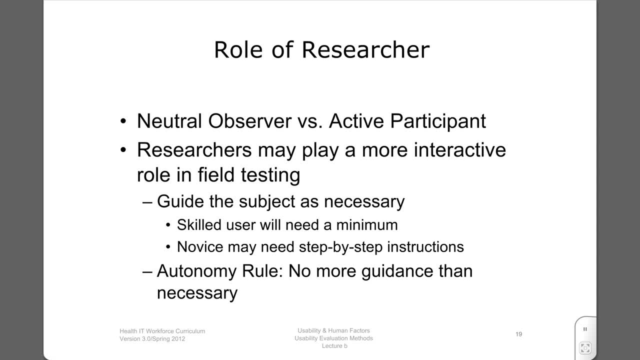 a complex task that you know will result in failure. What is the proper role of a researcher in a test situation? If your subjects are sufficiently skilled, then it is advisable not to interfere too much. Sometimes the role is regulated to encouraging the subject to think aloud. 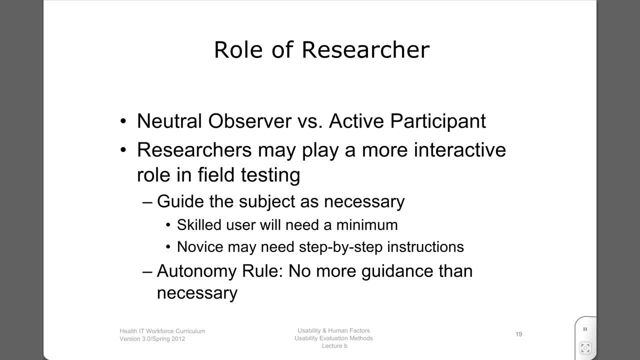 If a subject experiences difficulty with the tasks, then it is entirely reasonable to offer some assistance. We can't learn too much about the usability of a system if users can't even begin to complete the task. The goal is to provide as much guidance as is necessary. 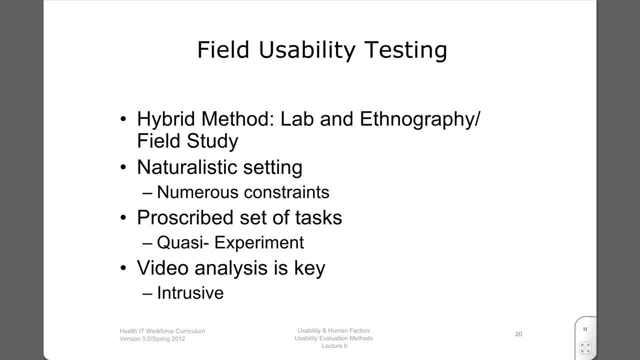 but no more than necessary. Most usability studies are conducted in a lab setting. Sometimes that's just an office of the investigator. Field usability testing can be rather challenging but very informative. You can study users in their naturalistic setting, whether it's 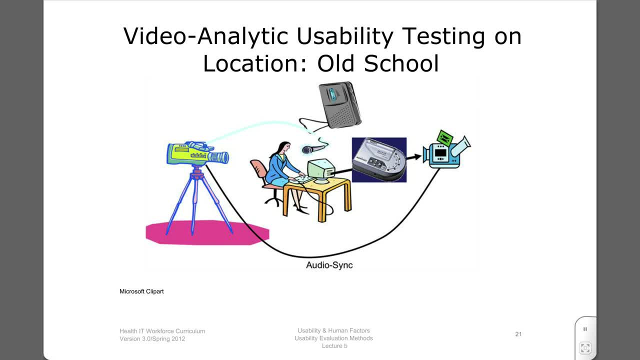 in a clinic or in a patient's home. Not too long ago, field usability testing was a difficult process involving a lot of technology. This typically included a video camera to capture the user and one to capture the screens. This often necessitated an analog. 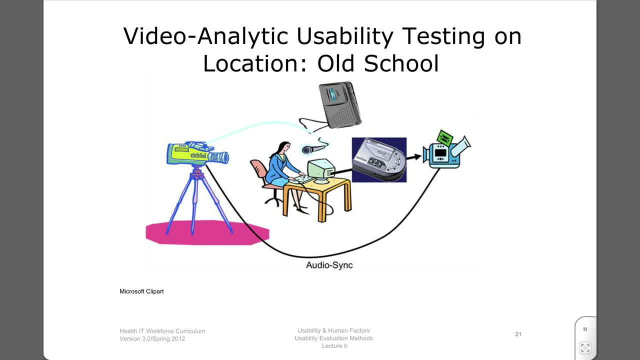 to digital converter, since it is very difficult to directly video record a screen. However, there are now video capture software programs that can easily do the work of this technology. This means one of two things: You bring a laptop to the field setting. 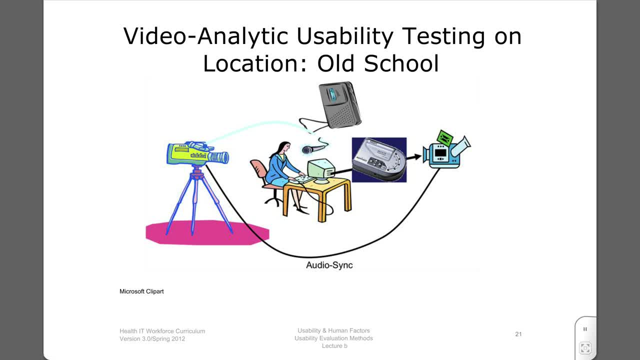 and you use it for the purpose of usability testing. The alternative is to install the software on a computer on site. This presents a range of problems, from securing permission to system conflicts, that make the process all that more difficult. It may be especially challenging. 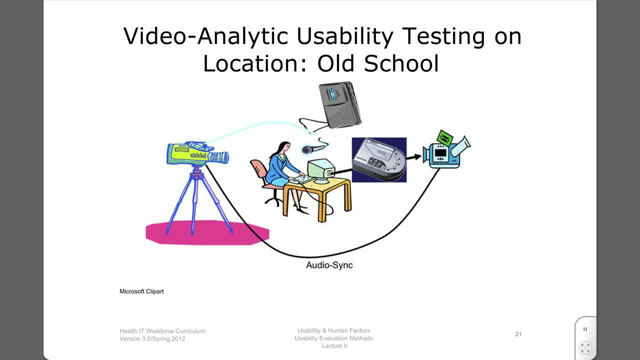 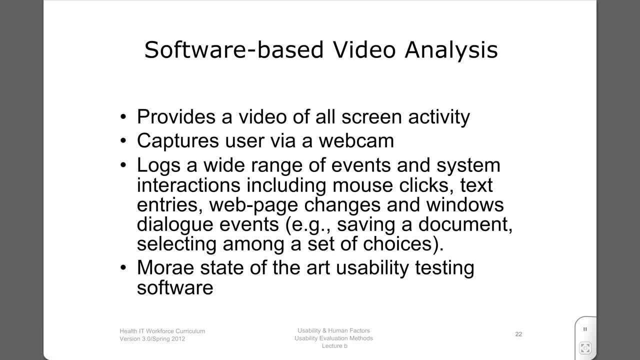 securing permission for installing software on a system that is used for viewing clinical data. There are a number of programs that support video capture and video analysis. Moray by TechSmith is one of the best. The software provides a video of all screen activity. 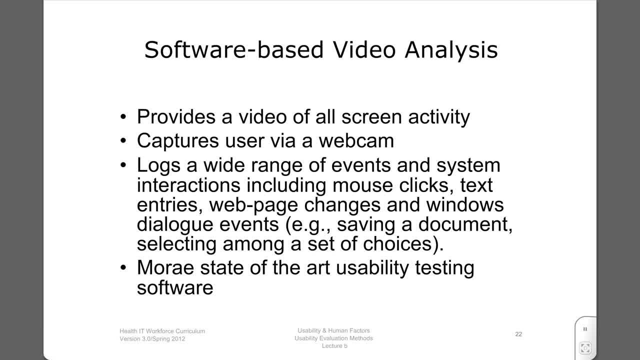 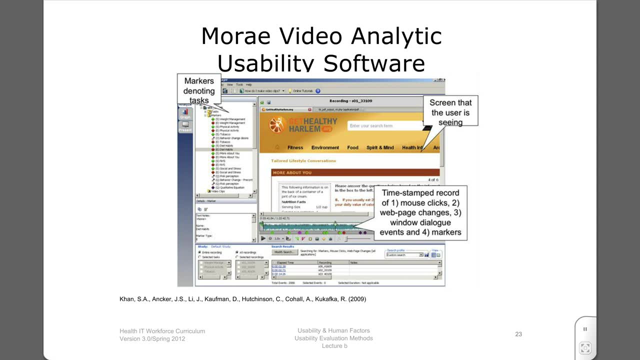 It can also capture the user via webcam, which can also record the think-aloud protocol. Such video analytic software can greatly enhance and expedite the process of video analytic usability testing. This is a screenshot of the Moray Manager, which is a powerful 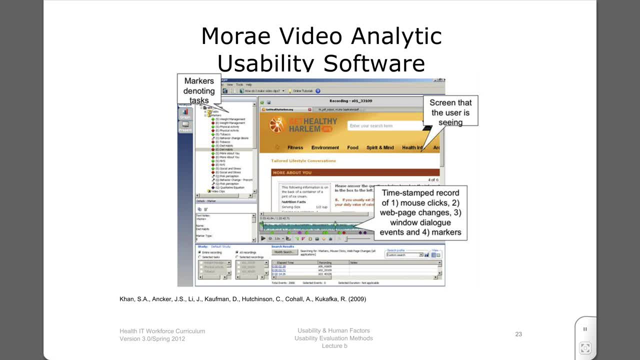 video analysis tool. A project consists of a set of users or usability sessions. These sessions can be broken down into a series of tasks and subjected to further analysis, such as the coding of problem types, The analytic tools log, a wide range of events and system interactions. 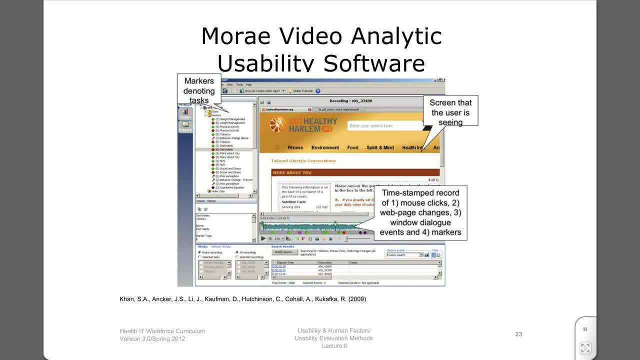 including mouse clicks, keystrokes, text entries, web page changes and Windows dialog events. We can compare performance of subjects across the same set of tasks. We can also compare performance problems and user errors, If a task resulted in performance problems and user errors. 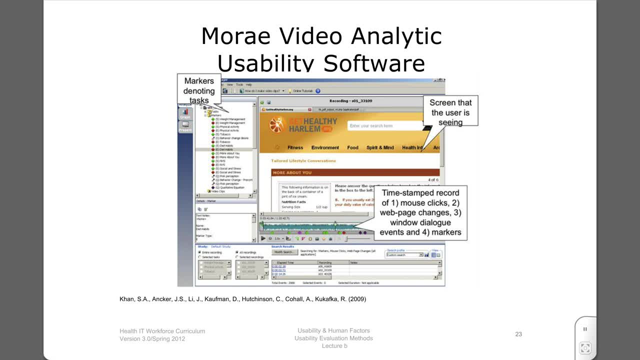 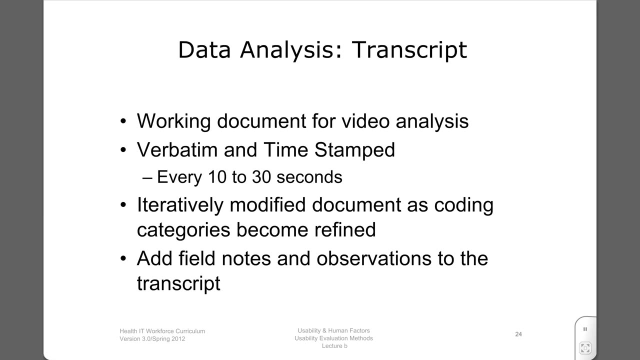 required numerous mouse clicks and longer than expected periods of time, then we know that there are usability problems. We can further scrutinize tasks at very fine levels of granularity to diagnose potential problems. A transcript includes the transcribed think-aloud protocol, which then: 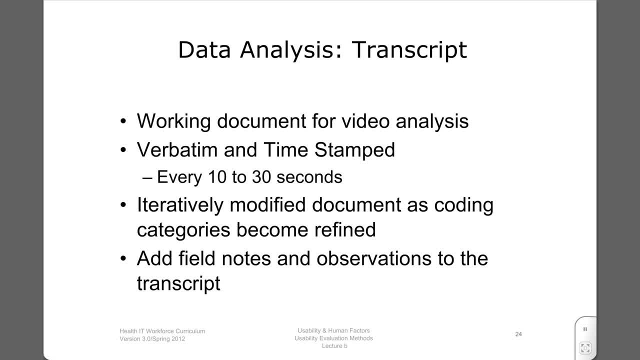 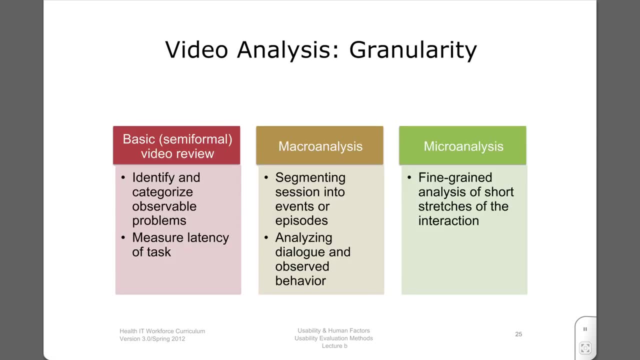 needs to be synced with the video. The transcript should include timestamps every 30 seconds or so. This serves to structure and index task performance. Video analysis can be performed at varying levels of granularity. At the most basic level, analysts may identify, categorize. 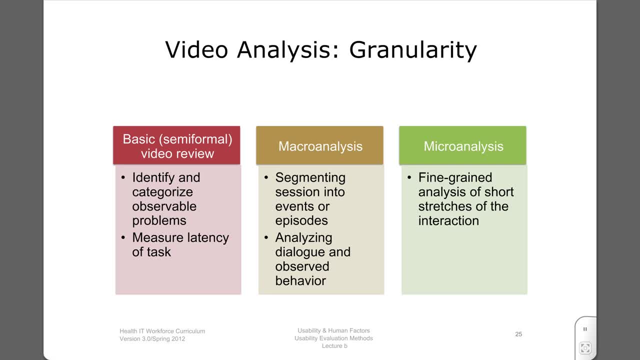 and quantify usability problems. A macro analysis involves an analysis of dialogue or the think-aloud protocol. Microanalysis is a much more fine-grained analysis and is very time-intensive. This latter analysis would be used to answer research questions and is not likely to be used. 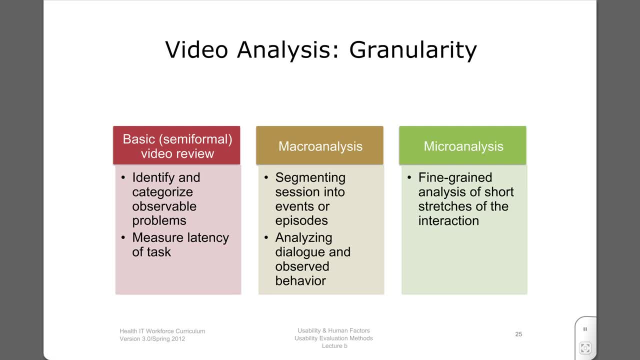 by usability analysts. The most basic level can be quite informative and will likely suffice for most purposes. The macro analysis can provide greater diagnosticity to the user, As suggested, although a microanalysis can yield substantial insights into usability problems and user competencies. 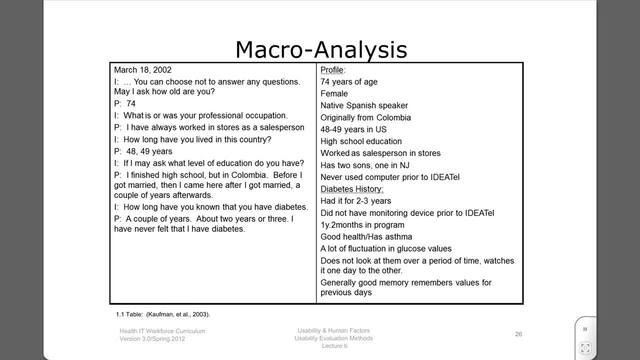 it is mostly a tool for researchers. This is a transcript of an older adult performing a set of tasks pertaining to a telemedicine system for patients with diabetes. There is a transcript of the first part of the testing situation, in which demographic data is collected. 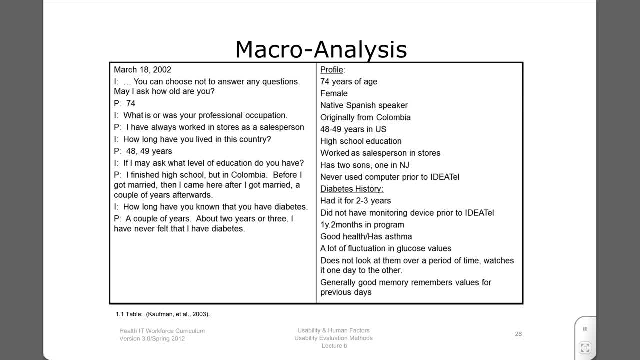 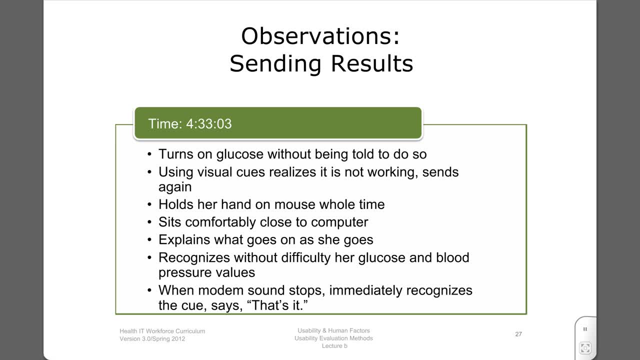 Although not in evidence on this slide, such analysis may include a description of the user's goals, actions and problems. On this slide, the user was performing a task in which she was able to execute the task without any difficulty. This slide has two. 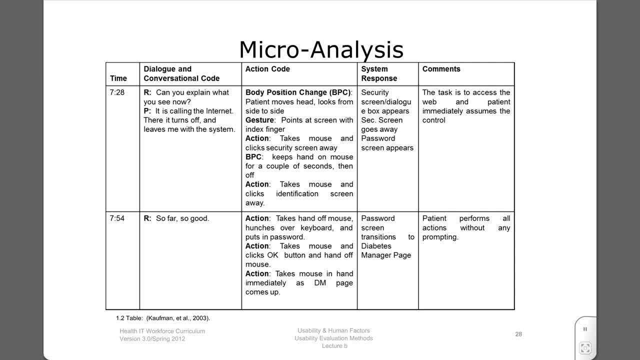 excerpts of a microanalysis. This is a very fine-grained analysis with moment-by-moment coding. For example, there is an analysis of every single action, verbalizations, changes in body movement for every hour of recording. A macroanalysis may necessitate: